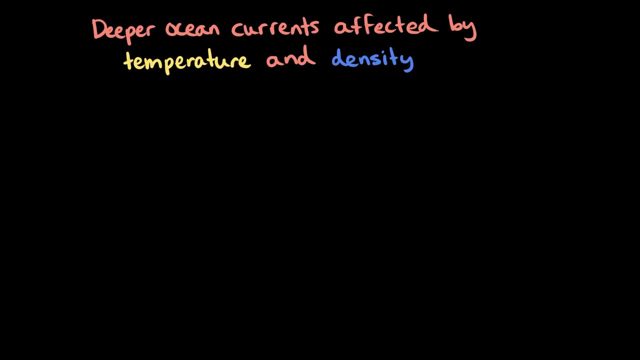 how that results in low and high pressure areas. Same thing with water, except that water density is affected by both temperature and salinity, which is a measure of how salty the ocean is. Cooler and saltier water is more dense, so it tends to sink, just like cool air, whereas warmer 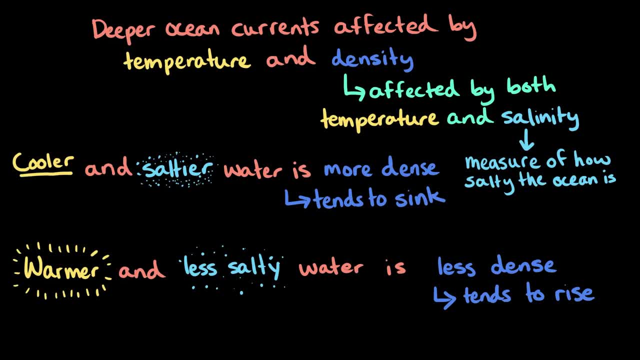 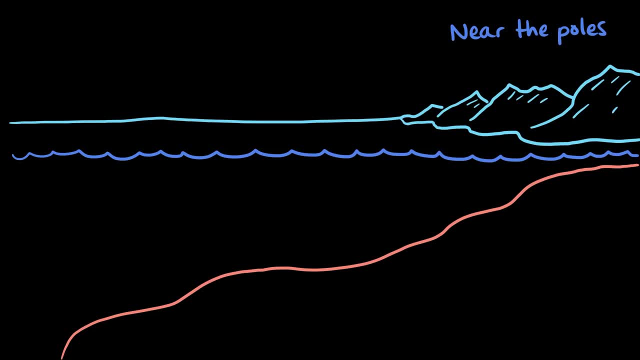 and less salty water is less dense and tends to rise, just like warm air. So with these deeper ocean currents water actually moves vertically or up and down. For example, water near the poles gets very cold. It also gets very salty because when sea ice is formed the salt can't go into. 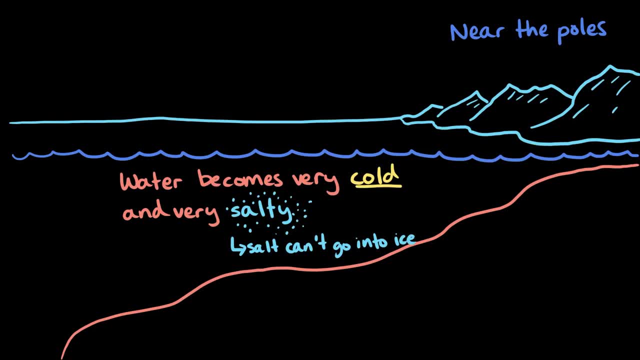 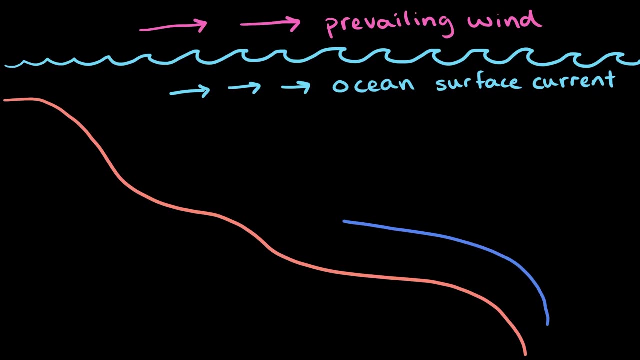 the ice. Instead, the salt stays behind in the water, and so the water gets saltier or more saline. Together, the coldness and salinity makes the water very dense, causing it to sink deep into the ocean. In other parts of the ocean, wind drags deep water up to the surface in a process called. 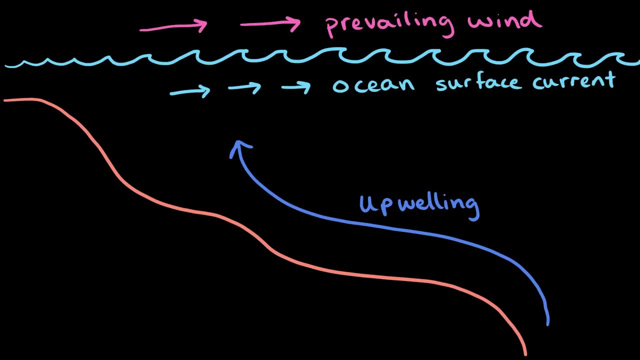 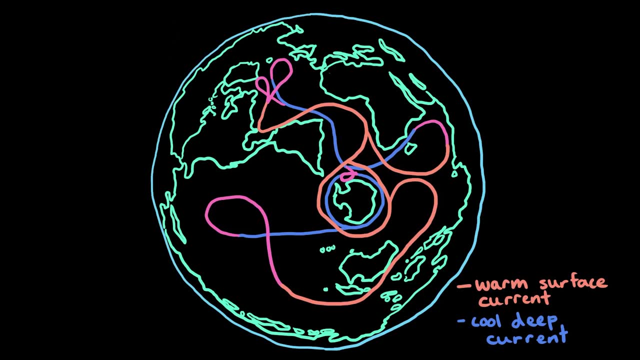 upwelling. These vertical currents are connected by horizontal currents at the surface and in the deep ocean. Collectively, this system of currents is known as the overturning circulation. You might also hear it called the global ocean conveyor belt. So here's.